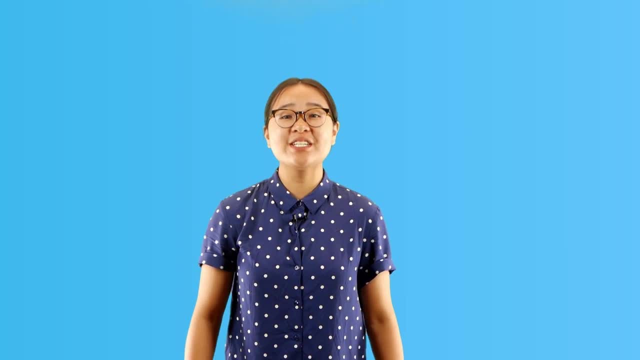 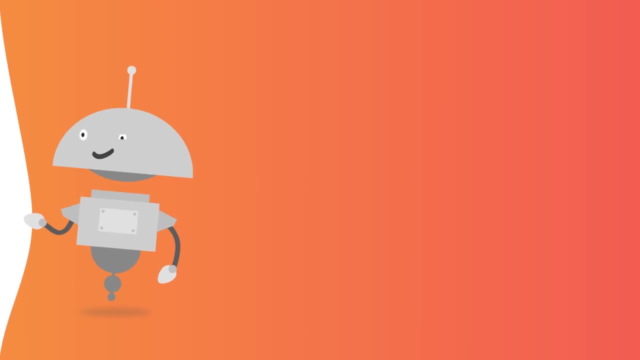 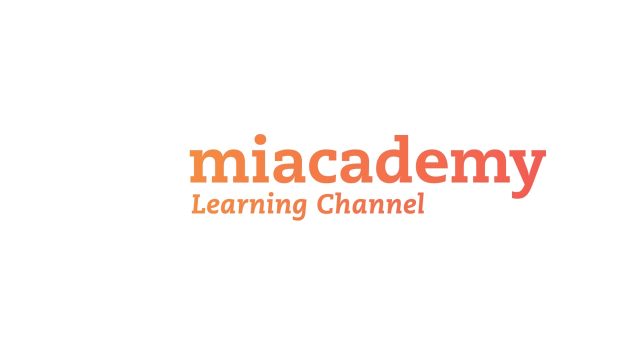 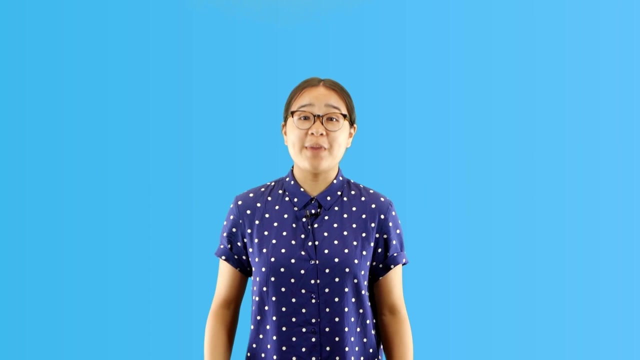 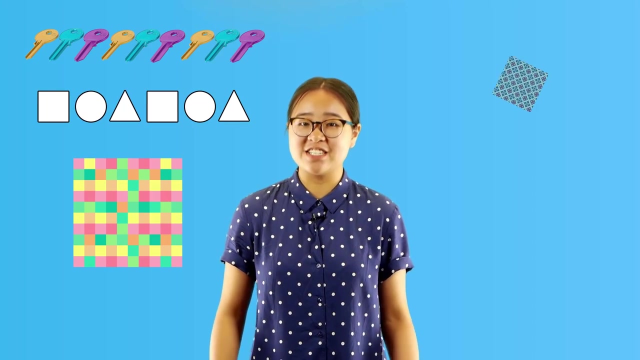 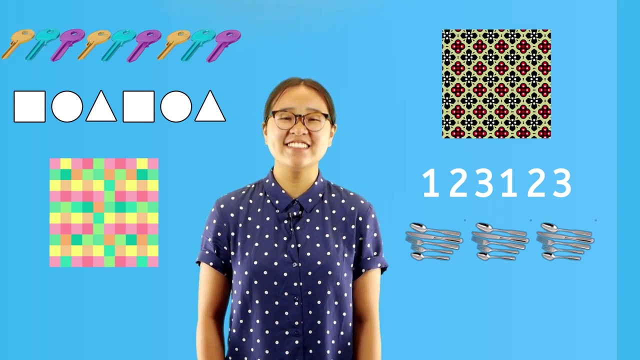 Hello and welcome to Number Sequencing. In this video you'll learn how to predict which number comes next in a series of numbers. Patterns are all around us. Patterns can be repeated items, shapes, colors, images or numbers. Sometimes a set of things are repeated to create a pattern. 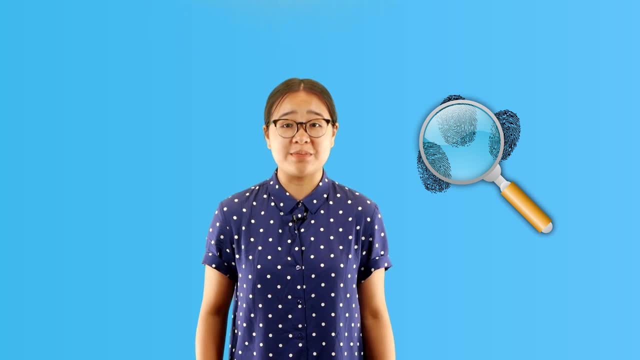 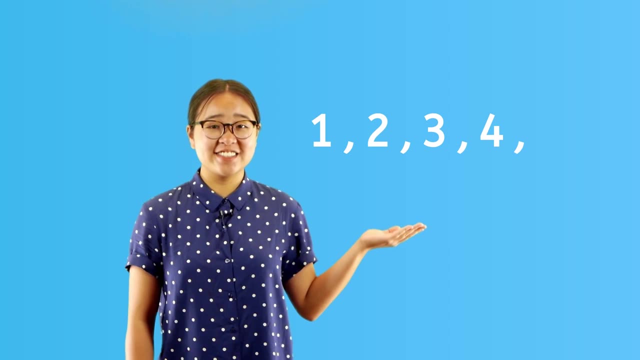 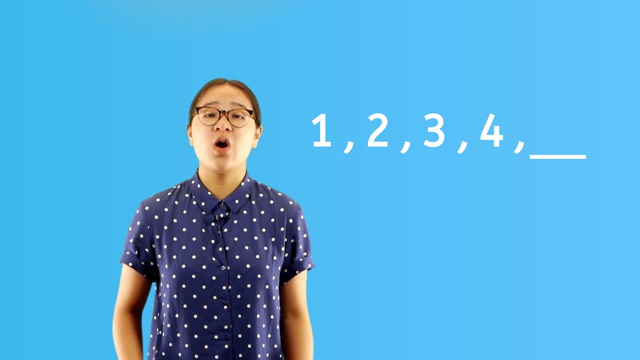 Number patterns are fun because you need to look carefully for clues to complete them. Here is a number pattern, or a sequence of numbers. What comes next? This is a fairly easy pattern because we count this one all the time: 1., 2.. 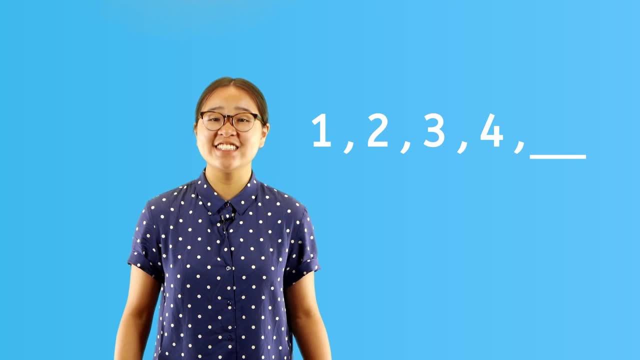 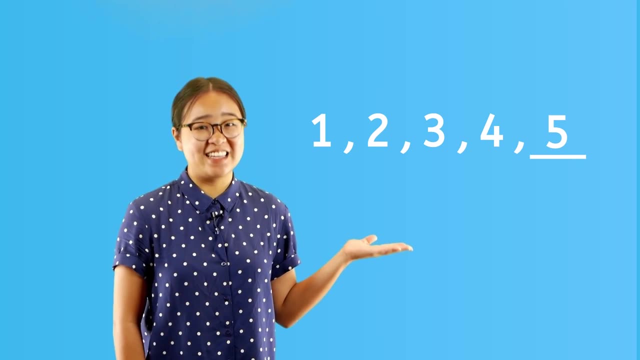 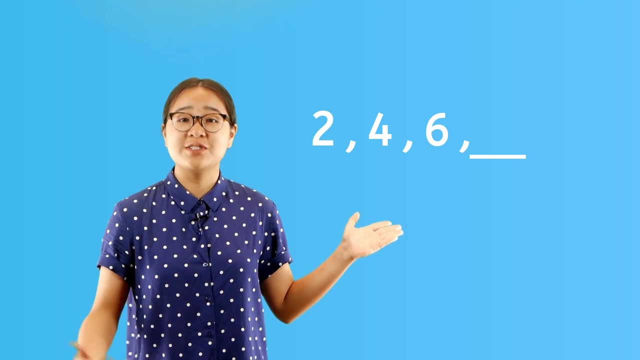 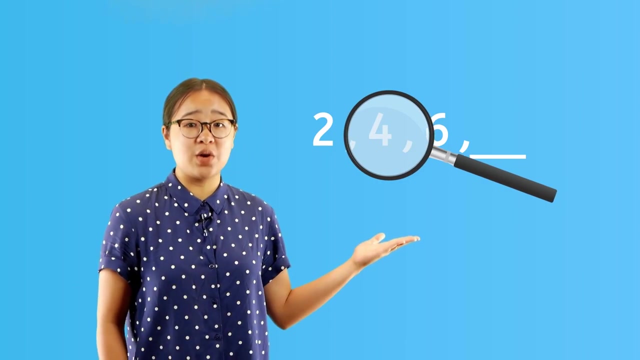 3., 4. And what comes next? Yes, 5.. Number 5 completes this pattern. Here is another one. What comes next? Let's see. We have 2,, 4,, 6. If you look for clues, we see that each number in this sequence is greater by 2..